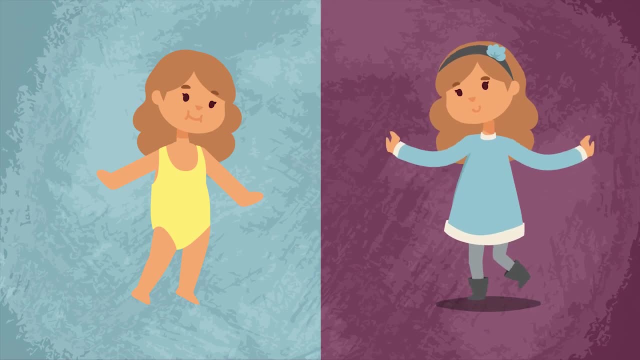 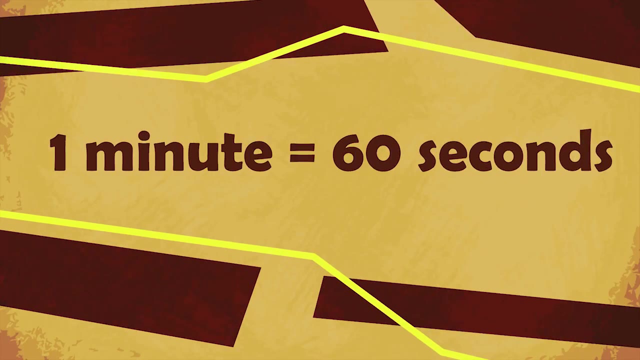 You might be able to hold your breath for one minute or hop on one foot for a minute. However, you would not be able to do these things for one hour. Just as there are 60 seconds in one minute, there are 60 minutes in one hour. 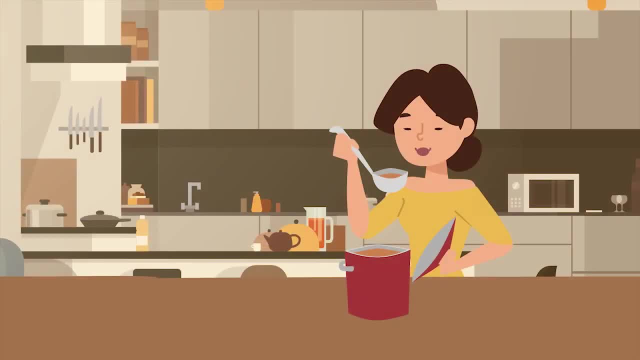 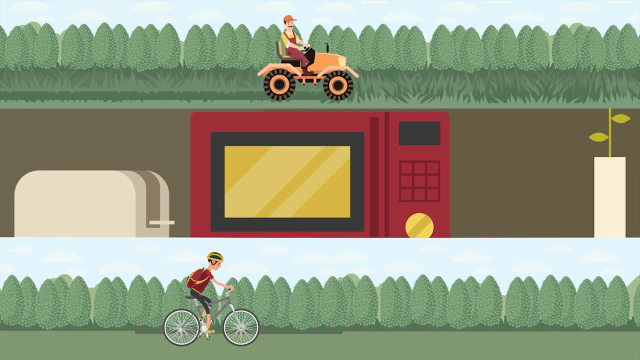 Many things can be done in one hour. Cooking a meal, taking a bike ride or mowing the lawn can take about an hour. Of course, some meals, bike rides and lawns may take less than or greater than an hour to complete. 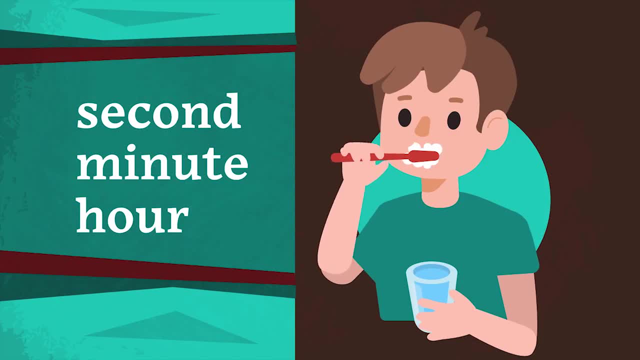 What unit would be most appropriate to measure the amount of time it takes you to brush your teeth? The second minute or hour? Hopefully you brush for more than a few seconds. Hours are too long. The minute is the best unit for measuring this amount of time. 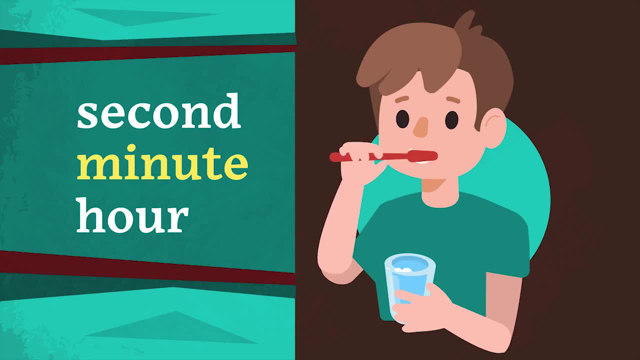 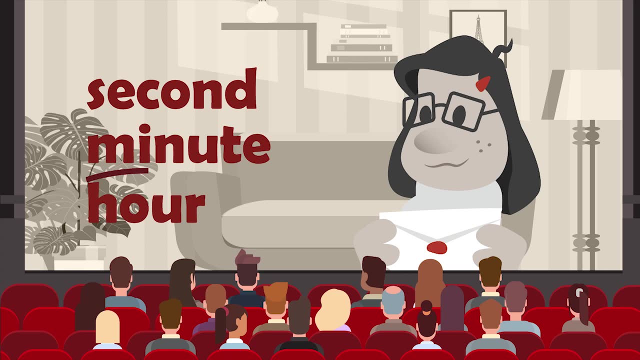 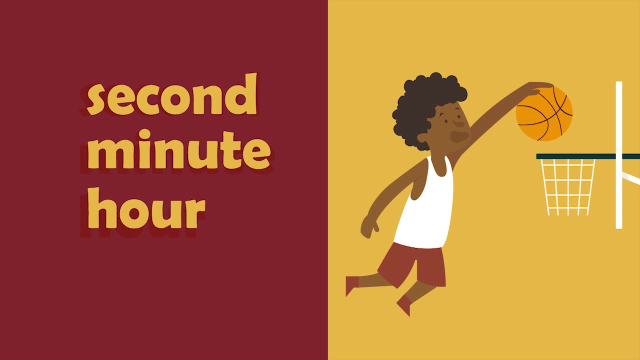 It should take you about two minutes to brush your teeth. What unit would be best for measuring the amount of time it takes to watch a movie? The hour is the best unit for this example. Most movies are about two hours long. Which unit is best for measuring the time it takes a basketball to go from a player's hands to the hoop? 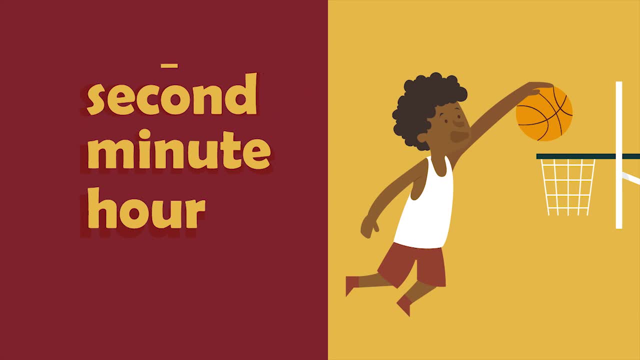 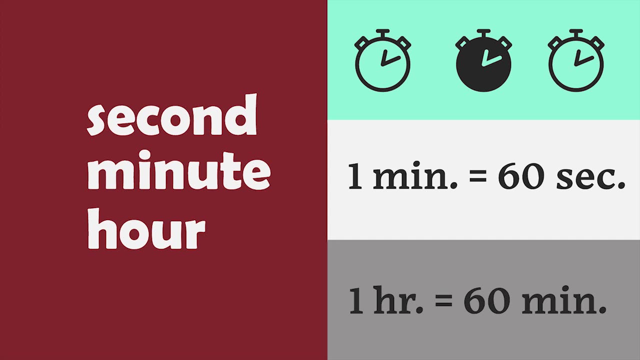 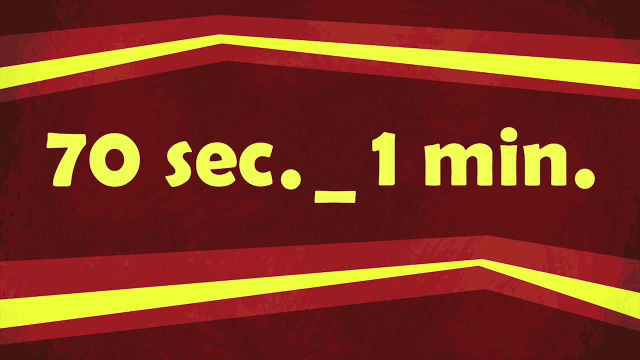 The second is the best unit of time. The third is the best unit of time to measure this brief action. Knowing how many seconds are in a minute or how many minutes are in an hour can help you compare amounts of time. For example, which is a greater amount of time, 70 seconds or one minute? 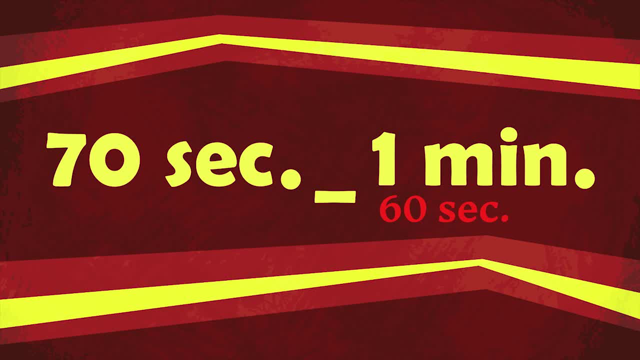 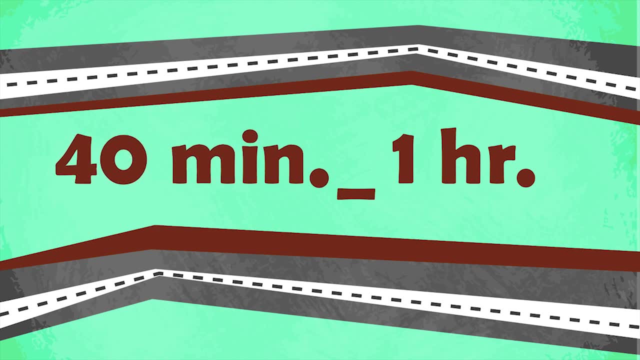 Since one minute is 60 seconds and 60 is less than 70,, 70 seconds is the greater amount of time. Which of these is greater: 40 minutes or one hour? Knowing that one hour is 60 minutes and 60 is greater than 40,, you can easily say that one hour is the greater amount of time. 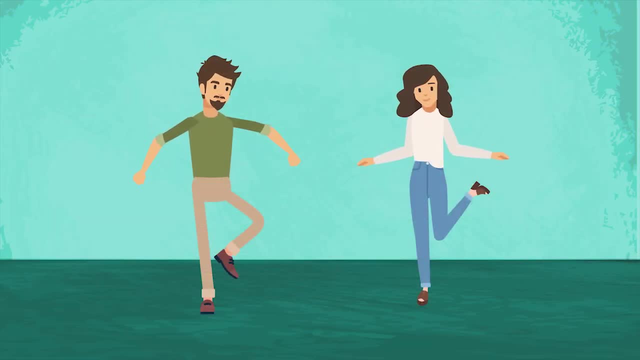 Two friends have a contest to see who can balance on one foot the longest. The first friend lasts one minute and the second friend lasts 85 seconds. Who wins the contest? Since one minute is 60 seconds and 60 is less than 85,? the second friend balanced longer and is the winner. 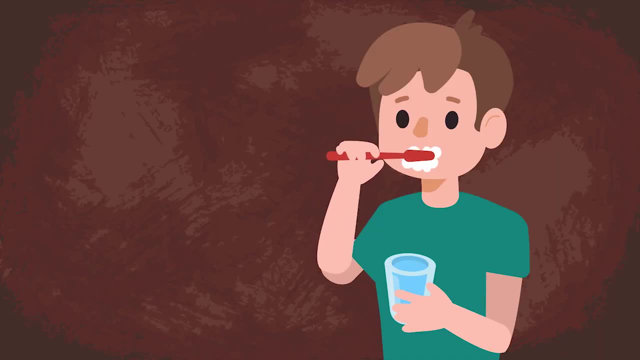 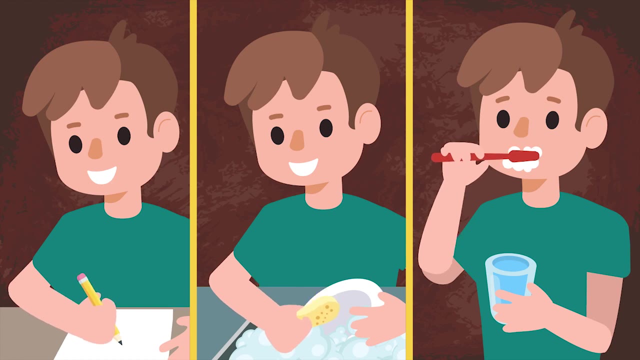 Time is an important part of everyday life, from brushing your teeth to completing chores or doing homework. Knowing how units of time relate to one another makes comparing them easier.